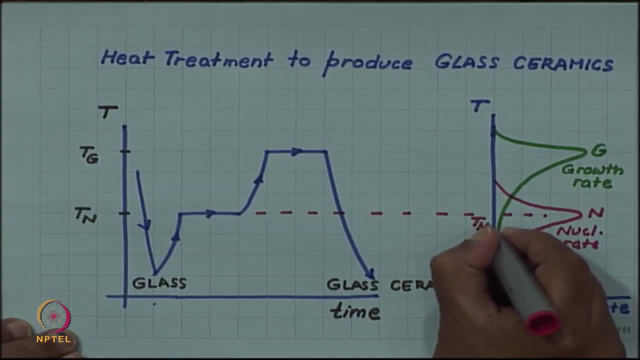 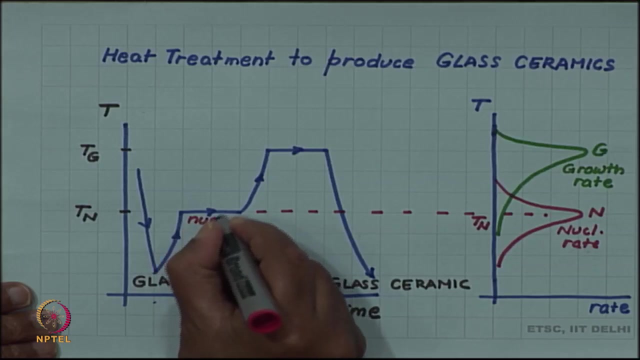 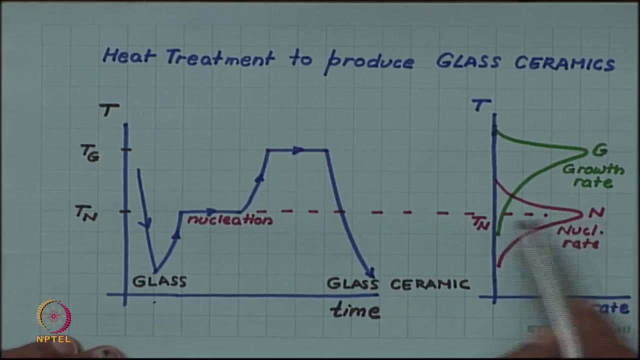 the nucleation rate is maximum. So several crystallites, several crystal nuclei, form during this period. This is a nucleation stage. However, if we continue at this temperature, the growth rate is very slow and the time required for formation of significant amount. 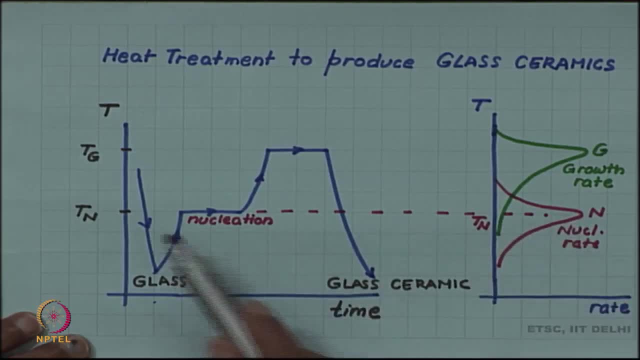 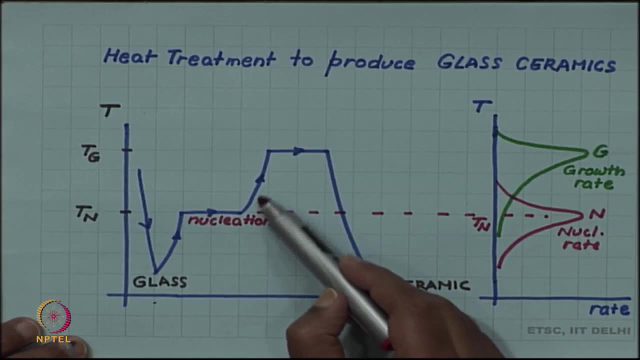 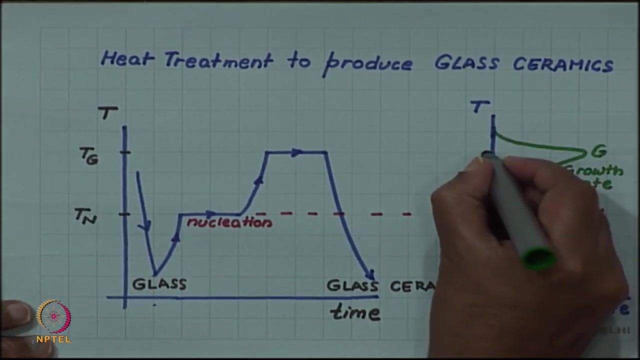 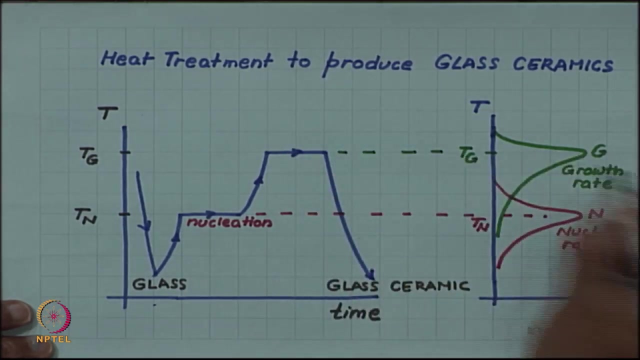 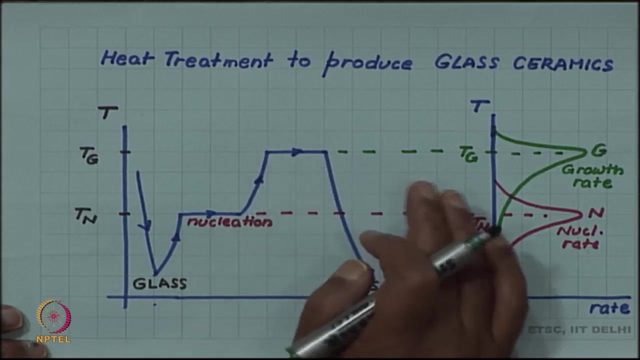 of crystal will be very large. So that is why a jump in temperature is given. after a sufficient number of nuclei are formed, temperature is raised to a value T g, which is the temperature at which the growth rate is maximum. So thus, whatever nuclei are formed at T n now, they start growing at a faster rate. 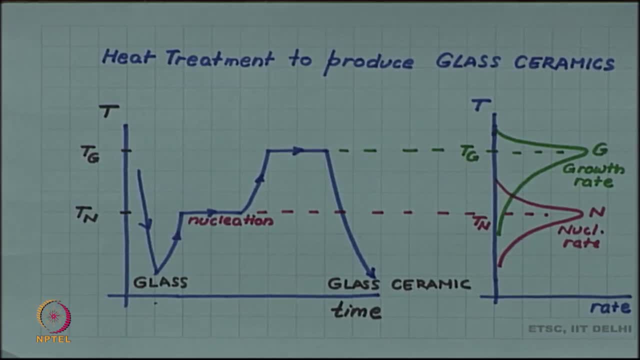 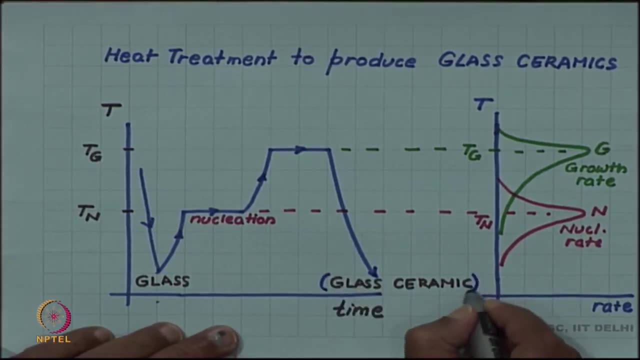 Finally, the material is quenched to form the so called glass ceramic. In this glass ceramic, in fact, it is not fully crystalline, it is actually glassy plus crystalline. So some glass matrix is also that plus crystal. delayed fulminating intelligent thermal pair. 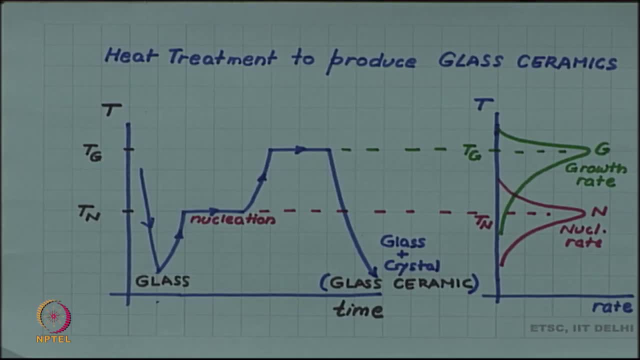 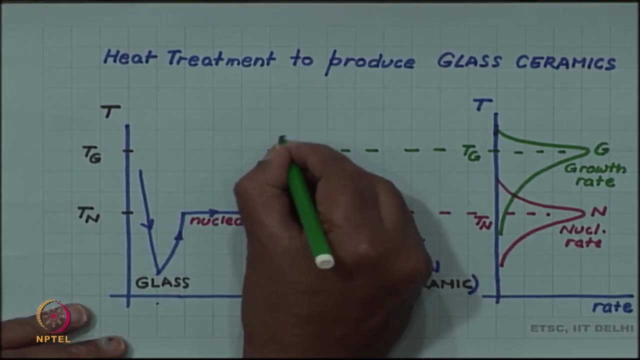 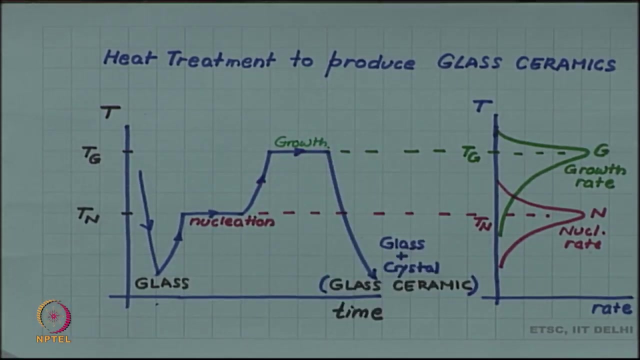 identification. One should also note that during the nucleation stage- this is for growth stage- and during the nucleation stage some heterogeneous nuclei, for example T i O t, is produced. It is not the only polymer stepping in which the glass matrix is scattered at Państlin Hallcoraaa. 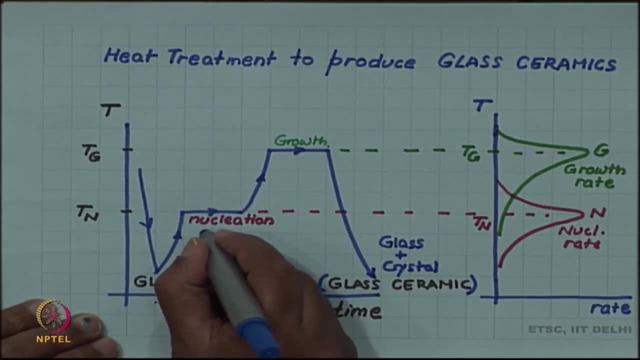 or aplic inform ultralnier voltage reaction. and one should also note that during the nucleation this has studied islands. this is the plane size of problems. PET branch she has used to nuclei, for example Ti O 2 precipitate and we have seen that heterogeneous nucleation. 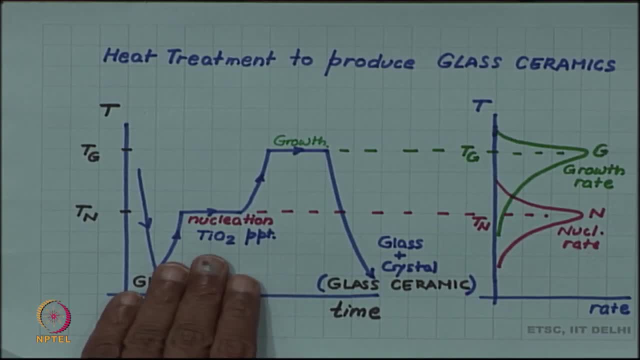 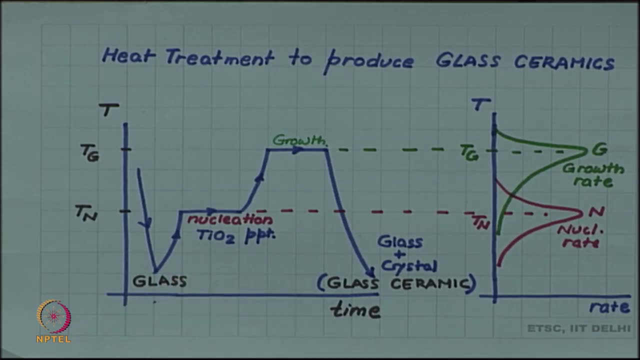 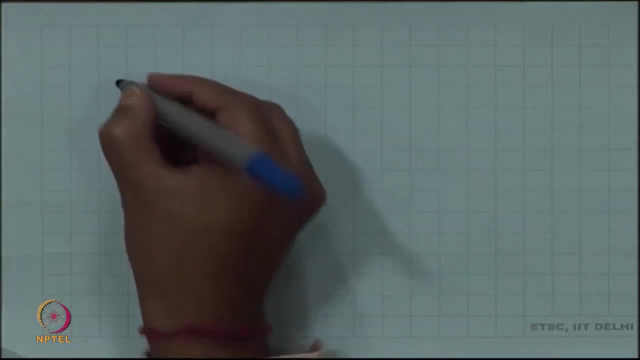 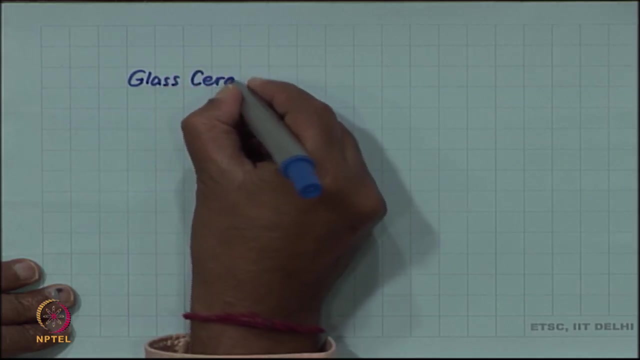 is easier than homogeneous nucleation. So these Ti O 2 precipitates form in the glass and they act as heterogeneous nucleation site which further enhance the nucleation rate. The ceramic produced by this heat treatment, the glass ceramic, is highly fracture resistant.